The history of child welfare in this country is, like most things, mixed back. There's a lot of progress. We have made a lot of progress, but there's still plenty of dark spots in there too. The first form of what we call foster care now appeared in New York in 1853, but it was not for. children who've been abused or neglected. It was for orphans or children whose parents could not afford to keep them. So less a removal situation and more a voluntary relinquishment situation. Now, that's 166 years ago, And the very next year, in 1854, there were more orphaned children. 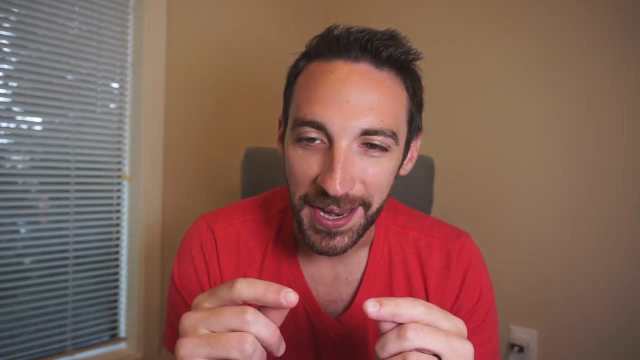 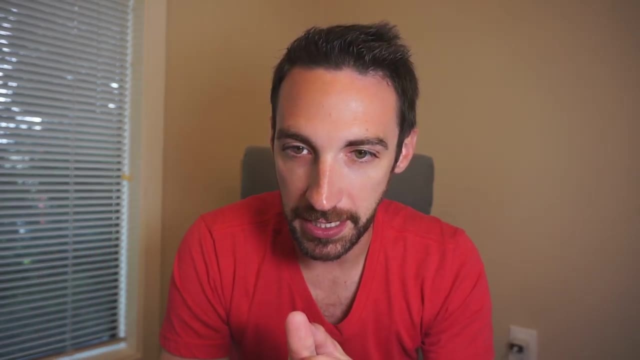 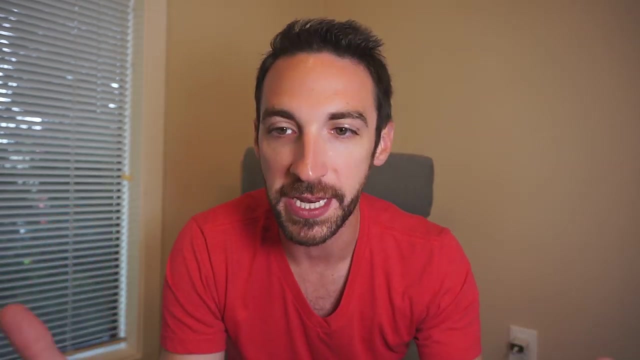 than there were families to welcome them. So this is not a new problem that we're working on. The first attempt to solve it was made by a fascinating fella named Charles Laurence. He was a very boring brace. He started putting orphans on trains bound for the Midwest because 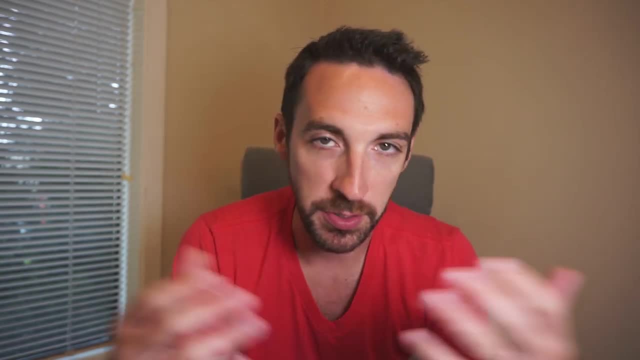 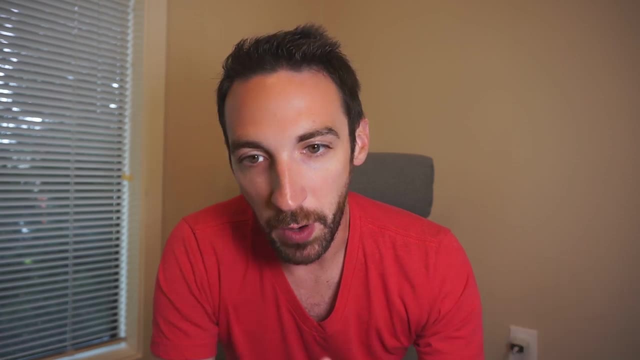 he thought homesteading families might like the chance to adopt children. There's always need for more help around the farm and many families had children, at least in part, for this reason. So Brace thought Midwestern families might jump at the chance to adopt half-grown children from. New York City. Interesting idea and it worked for some kids, but many more were never fully included in the family who took them and kept them a family. So we're going to talk about this in a bit, So let's get started. So first off the first orphan train, which was built in 1864.. So it was built in 1874. And then in 1874, so 20 years after the first orphan train. also in New York, a visiting nurse saw a little girl named Mary Ellen McCormick who was in really rough shape. 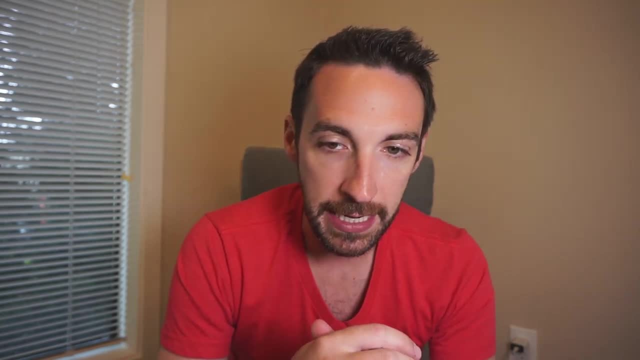 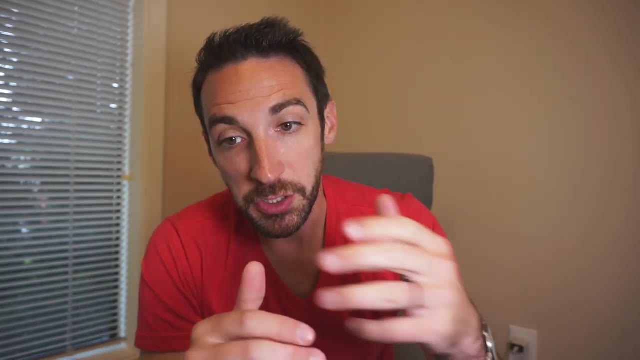 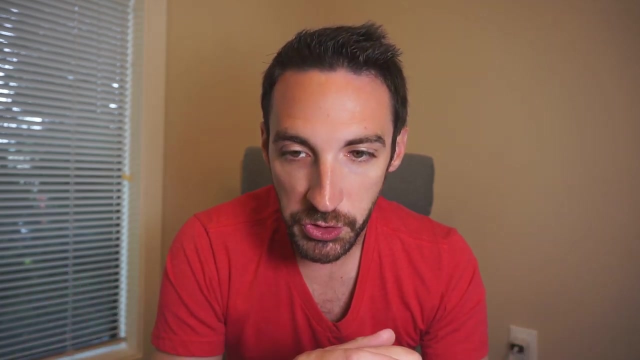 She was sick and dirty and bruised and malnourished And she, Mary Ellen, told the nurse stories about her mother abused her. So this nurse tried to intervene but found that there was no law enforcement law against mistreating children So there wasn't any direct legal recourse. But she was also quite 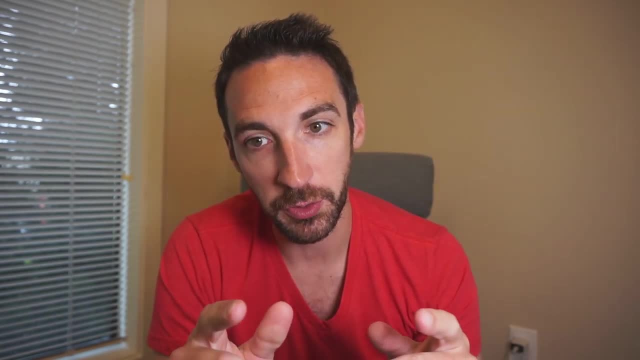 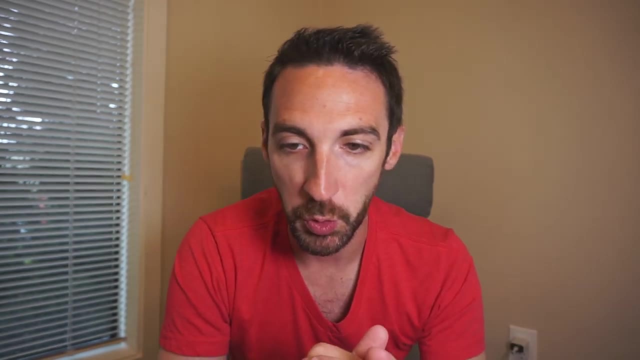 creative and managed to convince the Society for the Prevention of Cruelty to Animals to take up the case, And they argued all the way to the New York State Supreme Court, who ruled that it should be illegal to mistreat a child, And so Mary Ellen was removed from that. situation and placed with some of her relatives, And her mother was sentenced to jail for a year. Mary Ellen went on to live a very long and full life. She married and had children of her own and actually adopted an orphan girl. She died in 1956 at the age of 92.. 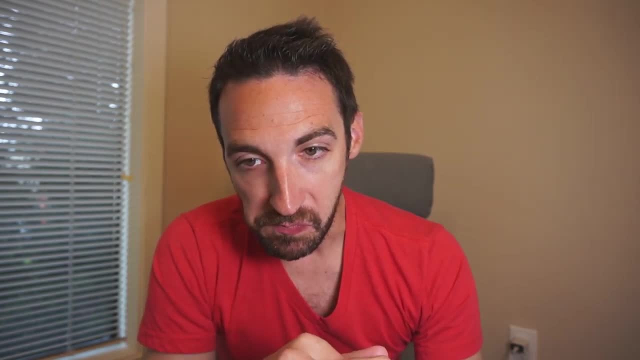 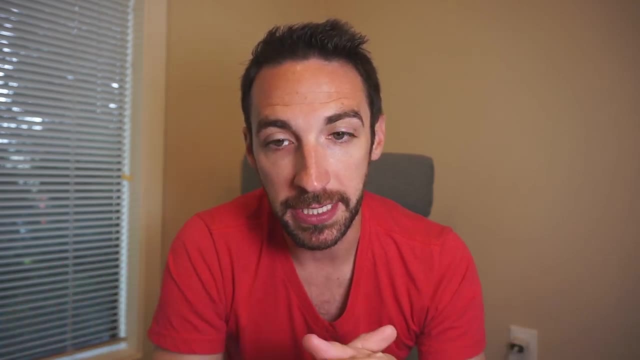 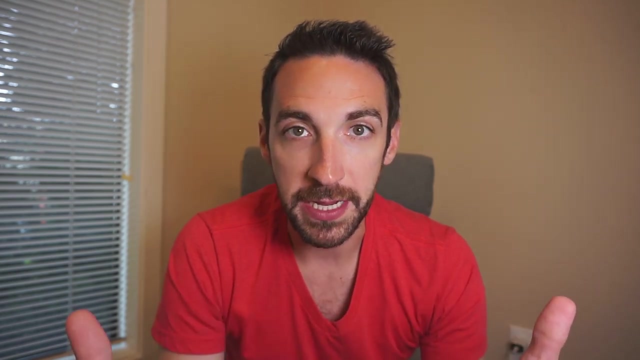 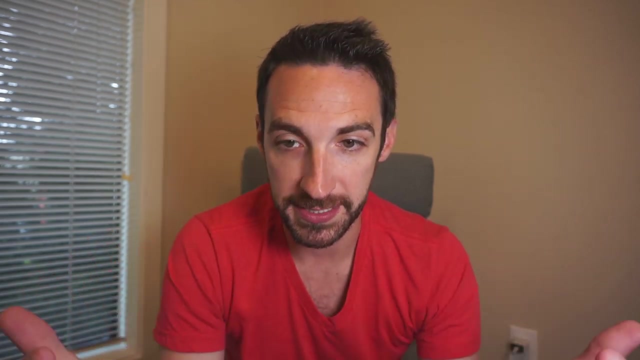 And then it starts to get dark From the late 1800s until 1978, roughly brighter the next hundred years or so. child welfare becomes weaponized as an instrument of attempted genocide of Native American peoples. Foster care and boarding schools were used as an attempt to remove Native children from tribes and raise them as white, with the intent of eliminating the tribes altogether over the course of a couple generations. This is one of the darkest stains on US history, and what brought it to an end was the Indian Child Welfare Act, which didn't pass until 1978.